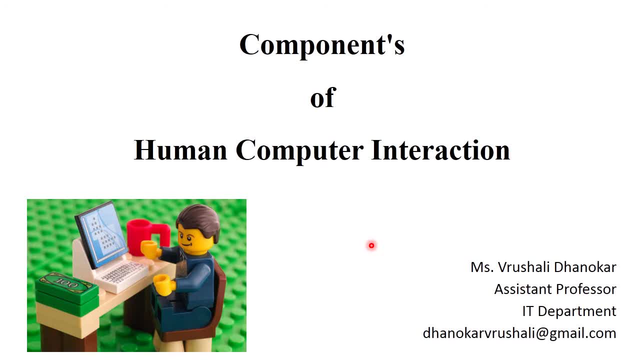 interaction. Right, Hope, so you guys understand all the points in more deeply. Okay so, let's So. in this video, we will learn about components of human-computer interaction. Okay so, let's see what is meant by components and how exactly this work. Okay so, in this video, the following: 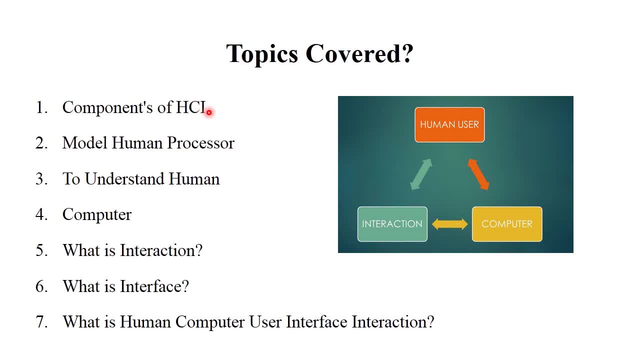 points are covered like components of human-computer interaction, model of human processor to understand human computer. what is interaction, what is interface and what is human-computer user interface Interaction? Okay, this, all points, will covered in this video. Okay, so let's see what is. 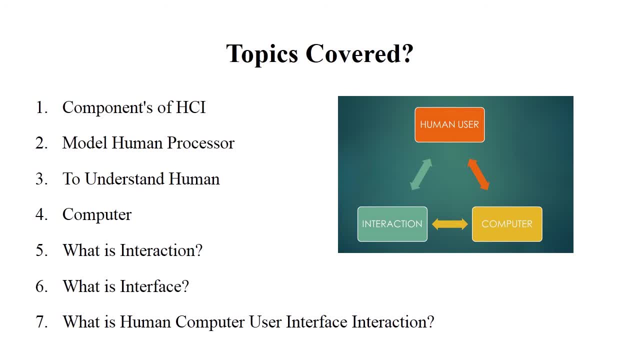 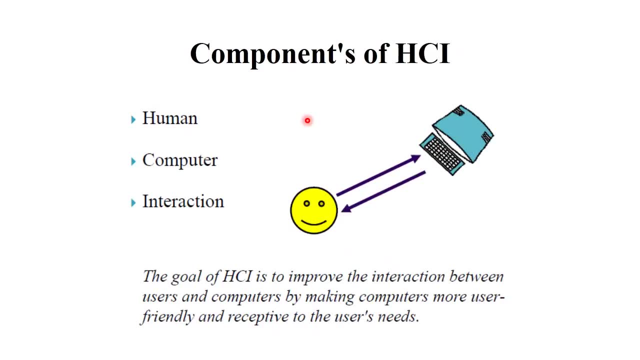 meant by components of human-computer interaction and how these components are exactly work. Okay, so see here the three main components of human-computer interaction. is human, computer and interaction. Right, by using these three components, each and every operations are. 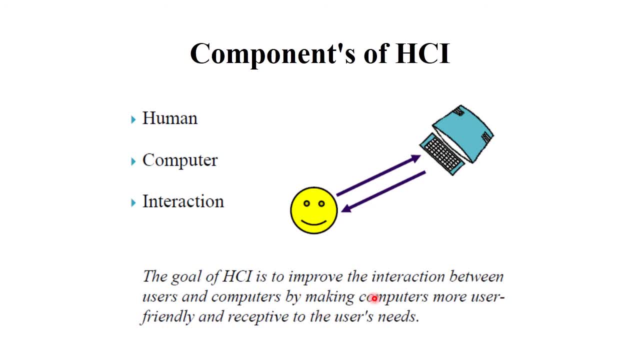 performed. The goal of human-computer interaction is to improve the interaction between users and computers by making computers more user-friendly and respective to the user's need. In a previous video I already explained goals and benefits of human-computer interaction. So for fulfill 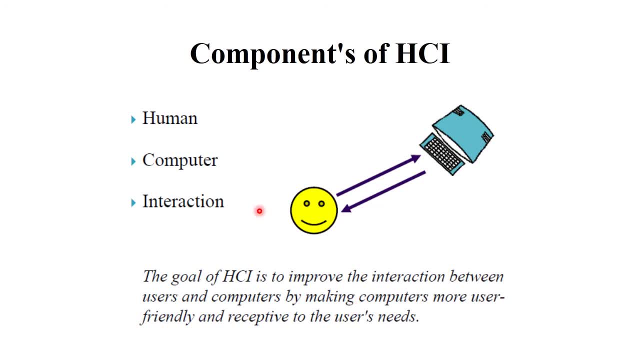 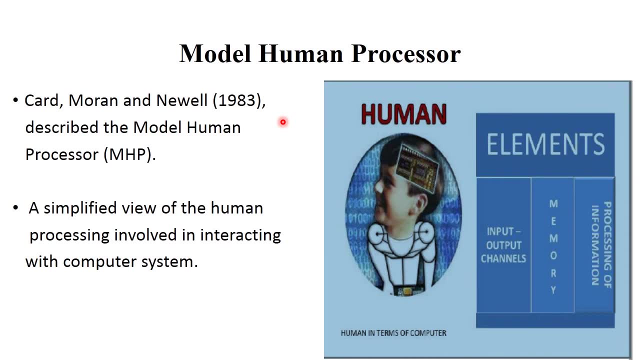 these goals and benefits these types of components are used. That is, human, computer and interaction. Okay, next, So let's see what is the model of human processor Now, when used. when you will study human-computer interaction, to understand a human is one of the essential part. Okay so, Card Moran. 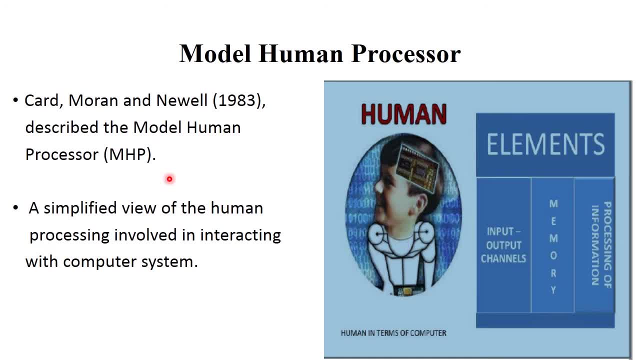 and Novel. This scientist in 1983 described the model of human processor. A simplified view of human processing involves in interacting with computer system. See in this diagram. there are three main elements, ie input-output channel, memory and processing of information. 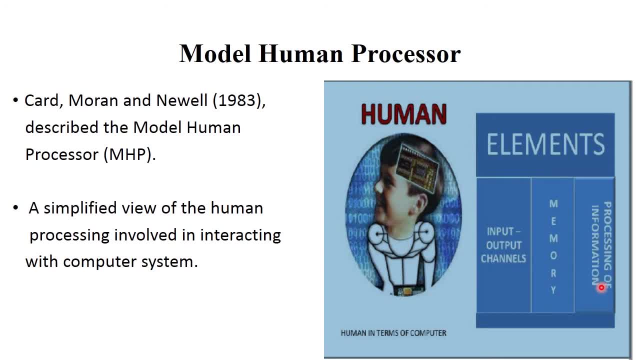 And what is the model of human processor? We are going to learn about human processor, So let's see the model of human processor. and what is human computer interaction? So information. there are three main elements of human processor. okay, we will provide input for. 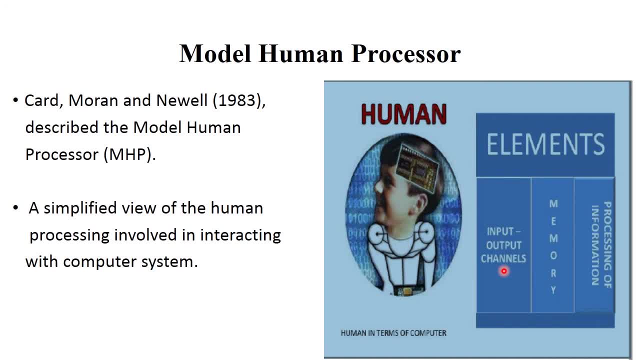 particular solution right and we also gets the output from this. so input and output is one of the necessary part of human right. human can store all the information in the memory. okay, there are various types of memory. this memory types we will learn in my next video. okay, so all this information. 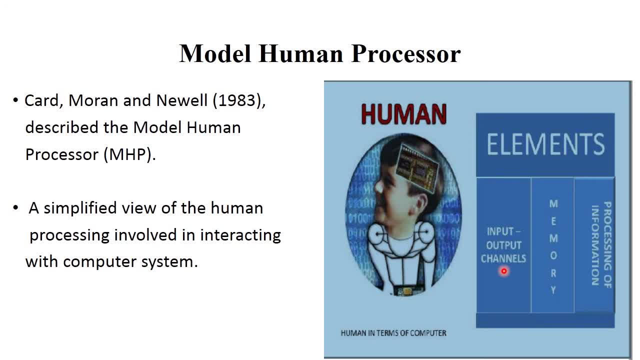 can be stored in memory and human processing all the information according to their requirements. okay, what exactly mean that? particular operations? okay, how exactly work this? all kind of information processing is done in human brain, right? so there are. this is a three. these are the three. one of. 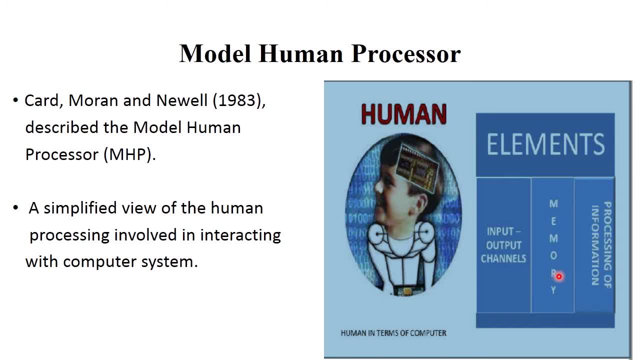 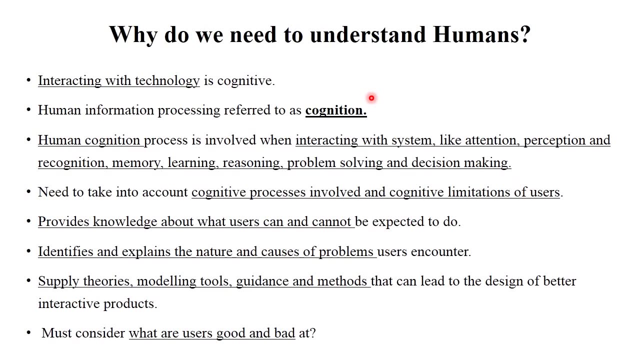 the most important. that is, input, output, channel, memory and processing of information, which is done by human right. so which is this is called as model of human processor? clear, ok. next, why do we need understand human? the human computer interaction, ok. so why do we need understand a human? so first interacting with 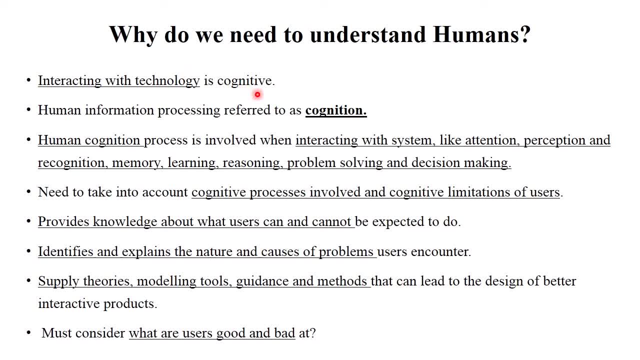 technology is a cognitive part. ok, human used mobile laptops, then computers, etc. all the technological gadgets are used to the human, used by human right. so interacting with technology is a cognitive way. the next human information processing referred as cognition. so what is meant by cognition? so human cognition is a process which involve interacting with system. 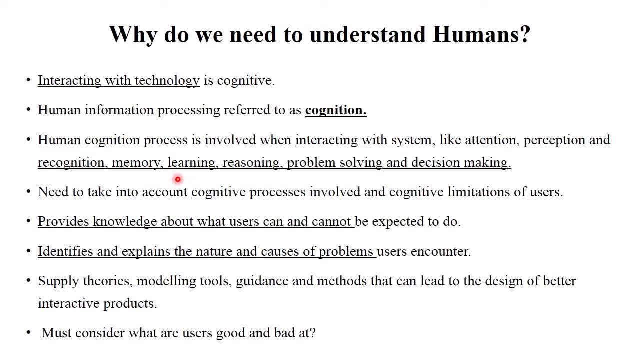 like attention, perception, recognition, memory, learning, reasoning, problem solving and decision making. human used computers and mobile laptops are used in the cognitive process. then how we are interacting with the computer ok, in a cognitive system. systems are used in the and laptops for their decision-making purpose, their problem-solving purpose. 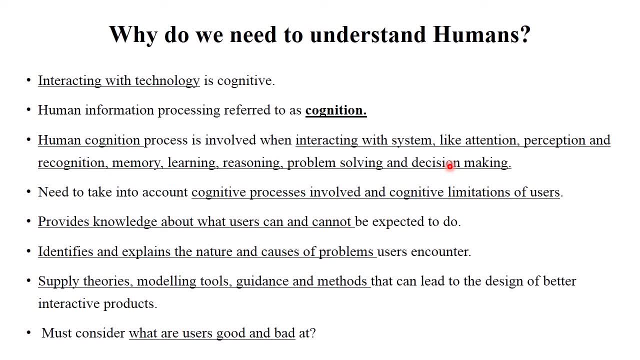 okay, that's why we need to understand humans: what exactly need of human and what exactly human want. okay, so all the needs and all the requirements of our human is fulfilled by human-computer interaction. right. it also need to take into account cognitive process involved and cognitive limitations of users, right. 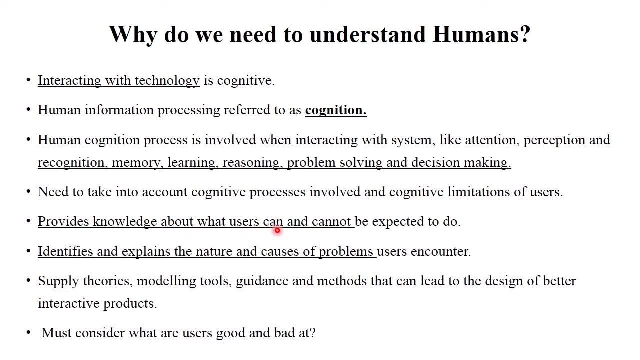 it also provide the knowledge about what users can and cannot be expected to do. if you need to know what exactly human want, then you need to develop this type of product. so for that purpose, requirements are clear, right. that's why we need to understand humans in more deep way. clear: it also identify, explain. 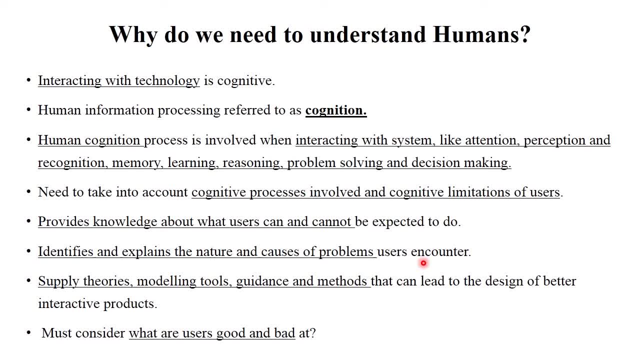 the nature and causes of problem users encounter. there are very social problems are arises and IT student, you need to solve all the social problems in technical way. This is one of the major responsibility in nowadays right? So that's why we need to understand the human. 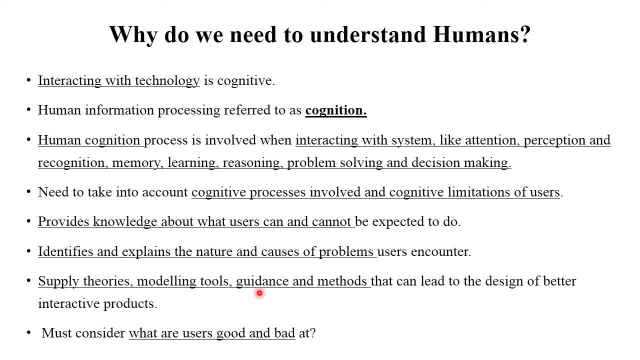 Also, there is supply theories, modeling tools, guidance and methods that can be lead to designer of better interactive products. It must consider what are the users good and bad? You need to understand what are the users are good and bad, Okay, And if you provide proper, 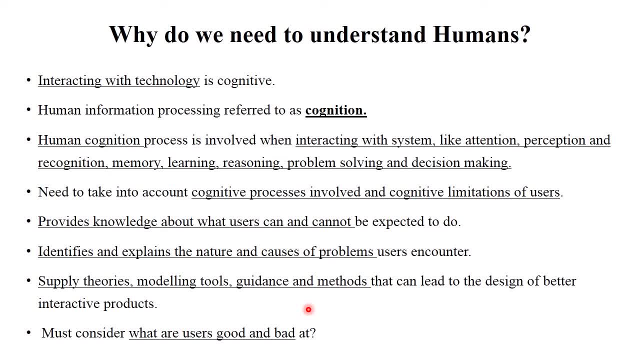 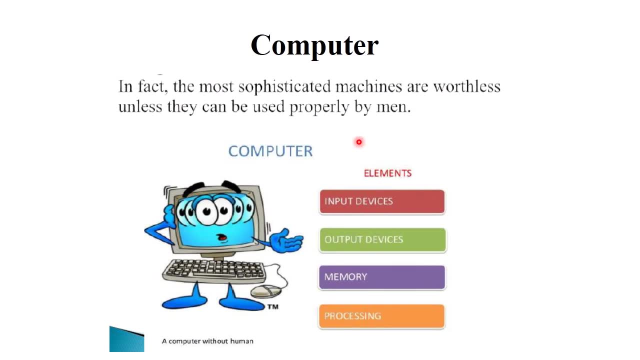 guidance and proper methods, developer developed a particular product which is useful for each and every people as per their requirements, Clear. That's why we need to understand the human. Okay Next. So what is mean by computer? We all are familiar with computer, In fact. 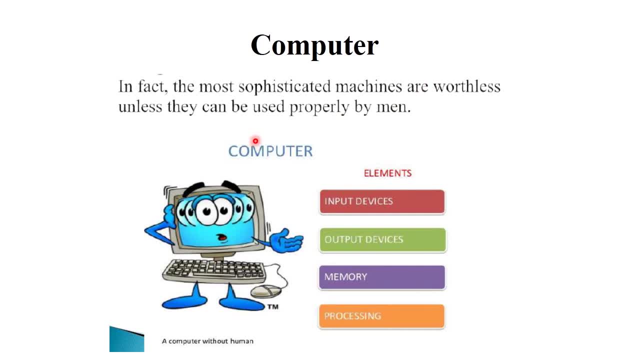 the most sophisticated machine are all of you. What is mean by computer? We all are familiar with computer. In fact, the most sophisticated machine are all of you. What is mean by computer? We all are familiar with computer. In fact, worthless unless they can be used by properly. okay, the elements of computers. 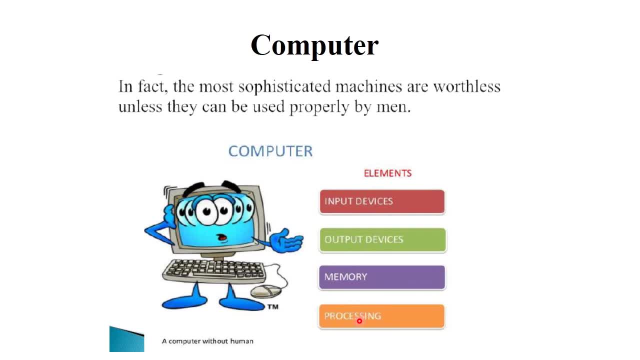 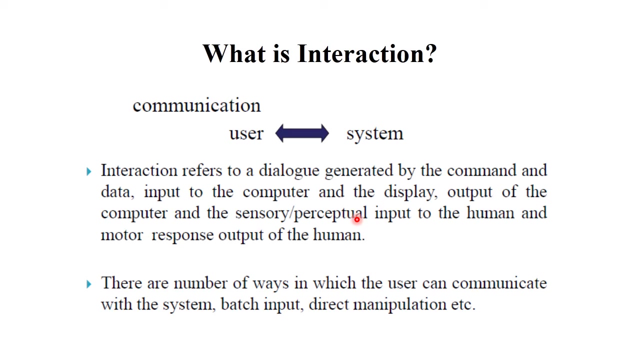 are input device, output device, memory and processing is similar to the human right. obviously, computers are also made by the humans right, so we all are familiar with all those elements. okay, so this is computer. next, what is mean by interaction? okay, interaction simply means computer or user. user used the computer for their decision making or problem solving. 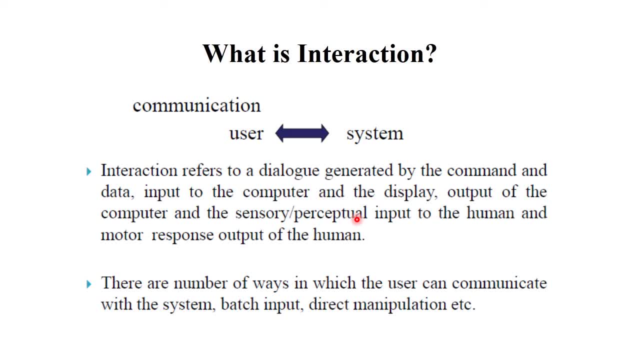 purpose right and computer gives the proper output. okay. so which is this is called as communication between user and the system? clear interaction refers the dialogue generated by the command data input to the computer and the display output of the computer and the sensory perceptual in input to the human and motor response output of the human. okay, when you provide 2 plus. 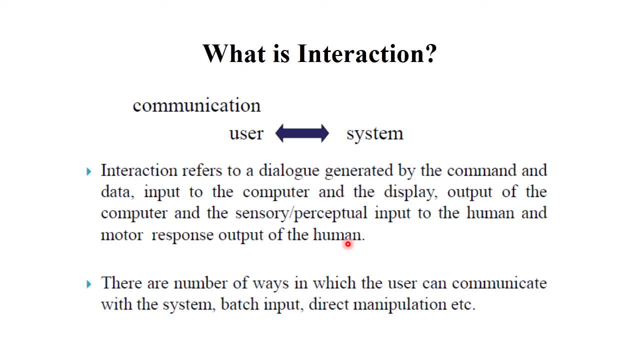 2 by using keyboard as a input to the computer. then computer provide 4 as a answer. okay, this is called input output part. okay, and for providing the input you used input output devices. okay, and computer provide the output to their screen. that is user interface. clear. there are number. 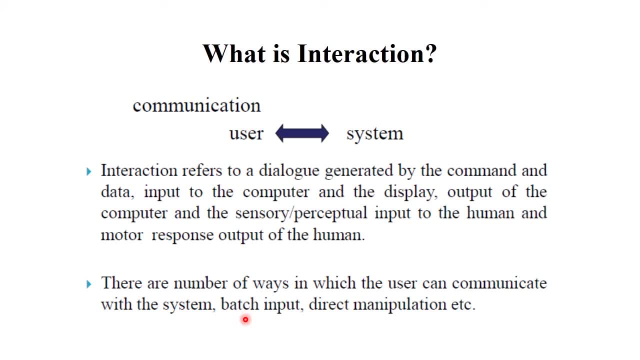 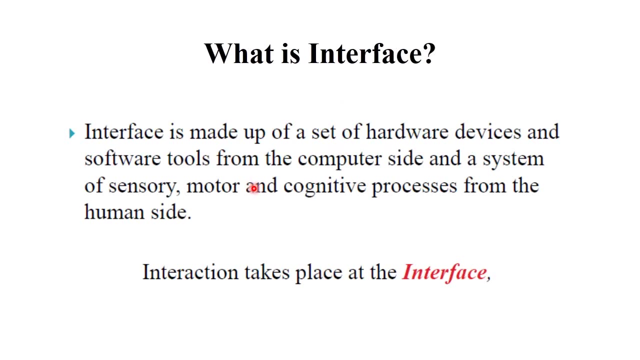 of ways in which the users can communicate with the system: batch input, direct manipulation, etc. clear, this is called as interaction. okay, next. next, what is mean by interface? interface means set of hardware devices and software tools from the computer side and a system of sensory, motor and cognitive process from the human side. okay, see here which is the. 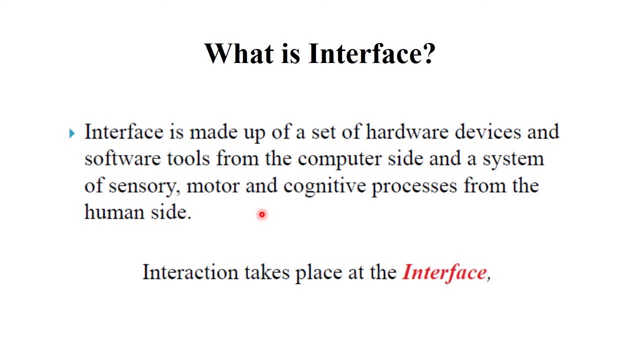 hardware part, that is CPU, mouse, keyboard, then a monitor. this all are hardware part. okay, user interacted with computer by using this hardware device. and what is the software part? software means operating system. or there are different types of applications are installed on operating system, right, for example Microsoft Word, PowerPoint, then browser. then again there are what surface book? 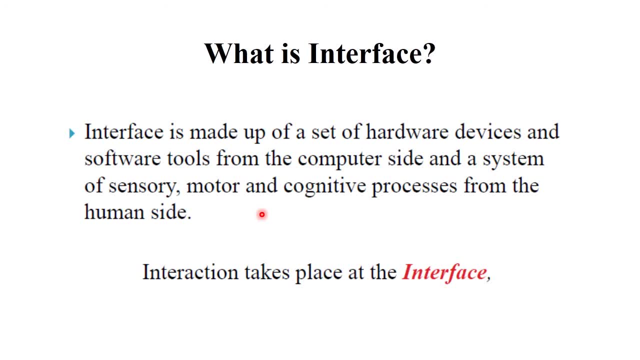 these all apps are interacted by the computer, right? so user interact those applications by using the computers or mobiles or laptops. this is called software tools. okay, so hardware device and software device or software tools are the interface of the computer. clear now what is the interface of human? 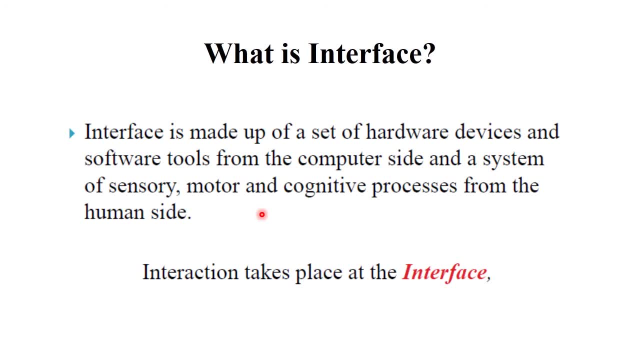 sensory, motor and cognitive process. these are the interface of human. human understand each and every part of computer right. human understand the how exactly every applications are work okay, and humans also get self-study regarding the each and every computers operations and applications right. so these are the interface of human, clear. so interface of